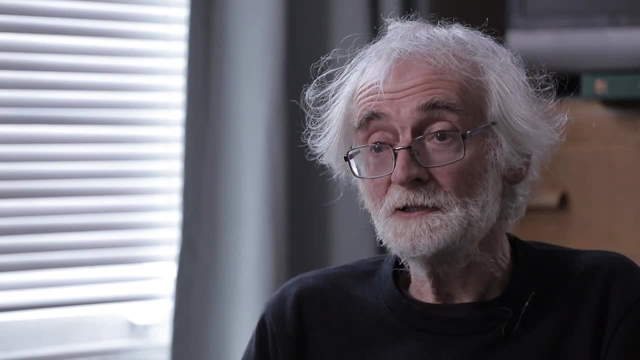 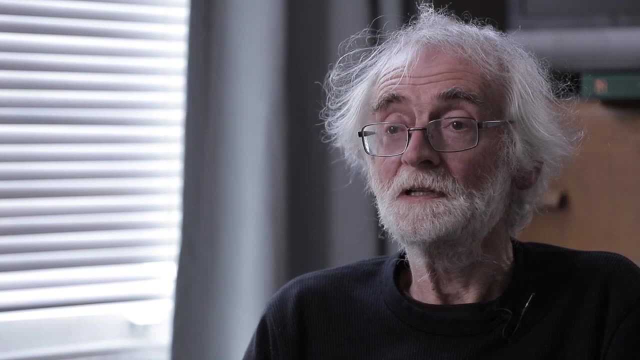 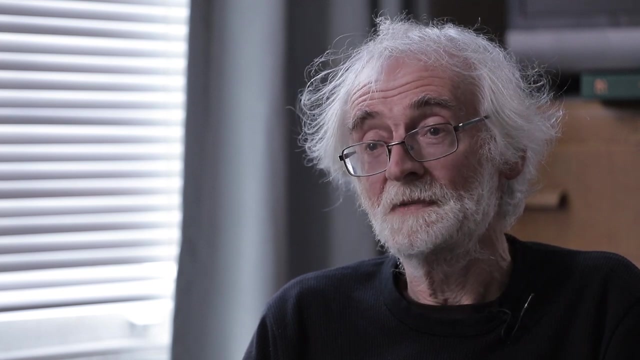 in. So, for example, the objects could be integers, the property could be divisibility by 10, and we ask: is this integer divisible by 10 or not? Now there is an easy algorithm to solve that problem. You just look at the last decimal. digit. If it's zero, you get zero. If it's two, you get zero. If it's three, you get zero. If it's four, you get zero. If it's five, you get zero. If it's six, you get zero. If it's. five, you get zero. If it's three, you get zero. If it's four, you get zero. If it's two, it's six. If it's six, you get zero. If it's five, you get zero. If it's nine: 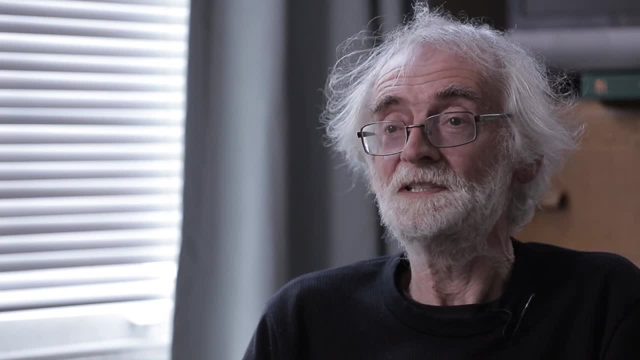 you can't be divisible by 10.. If it's one, it's divisible by ten. If it's eight, you get zero. it's divisible by ten. If it is one, it's divisible by ten. If it's not zero, it's not divisible by ten". 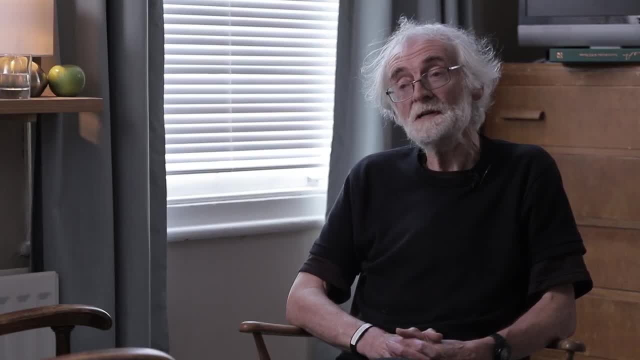 So that is an algorithm which solves this problem. and we say that a problem is noticeably single letteran algorithm to solve it, or see received in caption 6.9, an algorithm being a veggies finite repertoire, following the principle of the Deus es chiaro muscle. 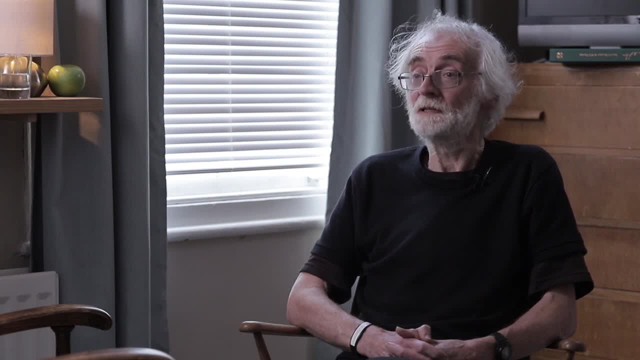 et Hua non smetataева. it�s the same as readingツ最後 мама et adervices gives the correct answer. It must, after a finite number of steps, produce the correct answer: yes or no. Now, what I would like to do first is give you an intuitive argument. 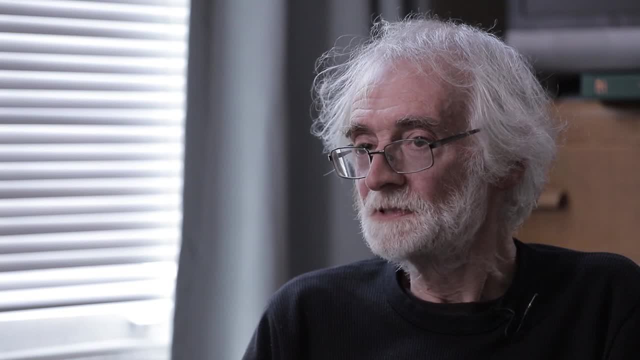 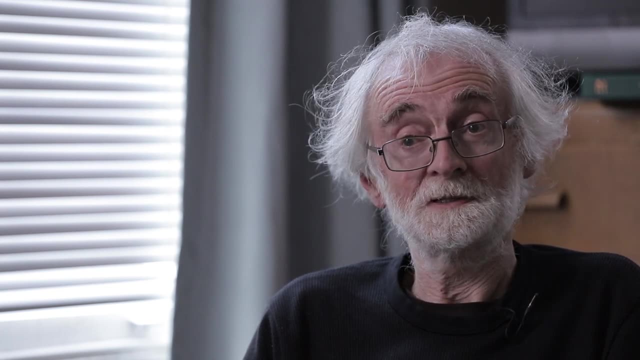 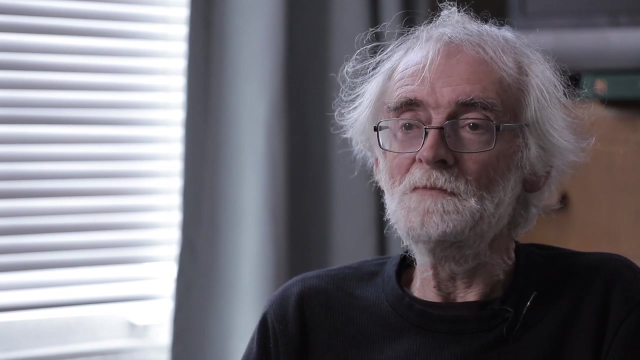 as to why one might expect some problems to be undecidable, And the reason is that there are infinitely many problems one can ask and there are infinitely many algorithms one can describe, But the infinite number of problems is bigger than the infinite number. 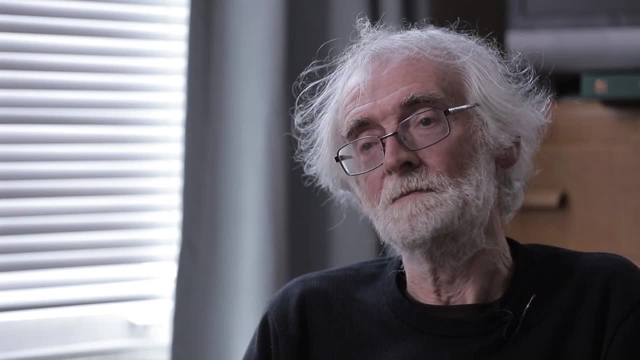 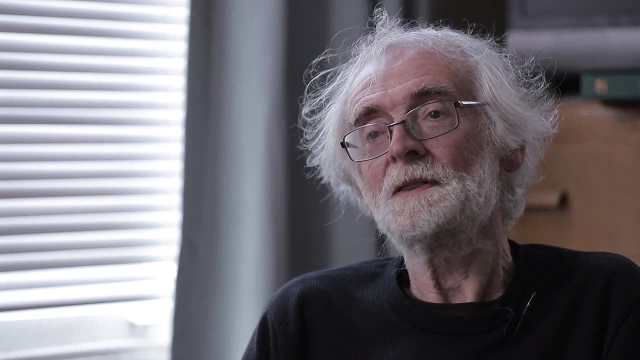 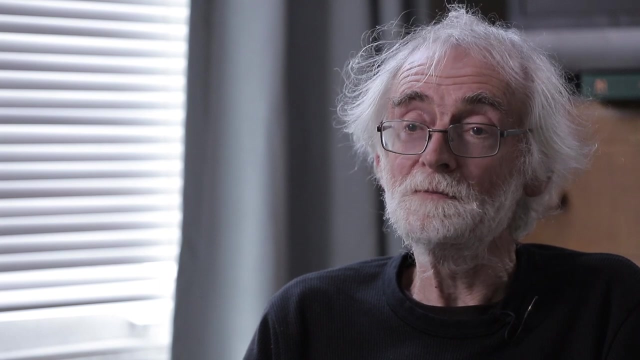 of algorithms, so there simply aren't enough algorithms to solve all the problems. Now, the algorithms form a set that is countably infinite. That's mathematical jargon. and for saying that you can form these algorithms into a list, There's a first, a second and 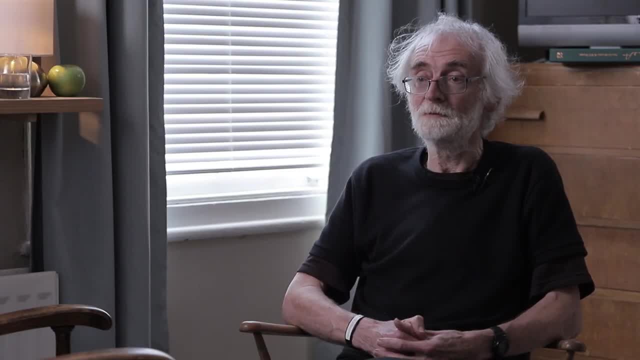 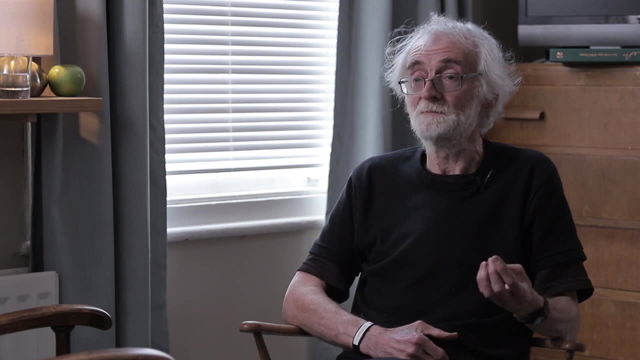 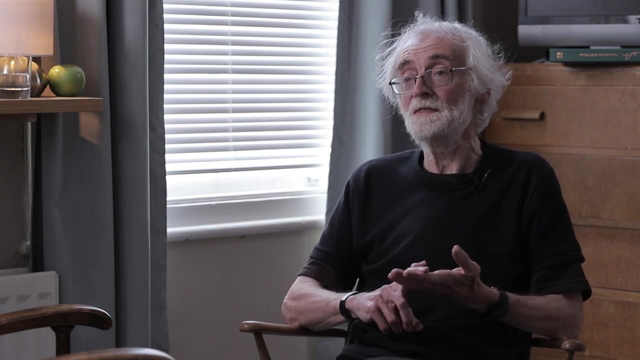 a third member and so on, And all algorithms will eventually appear in this list. You can do this with the integers, for example. I can list all the integers. Now I can't go one, two, three and so on, because then the negative numbers and zero are left out. But 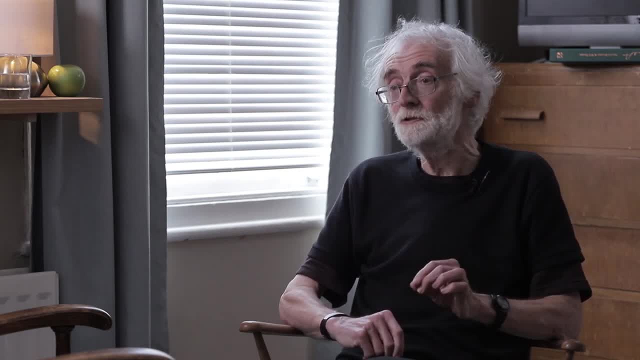 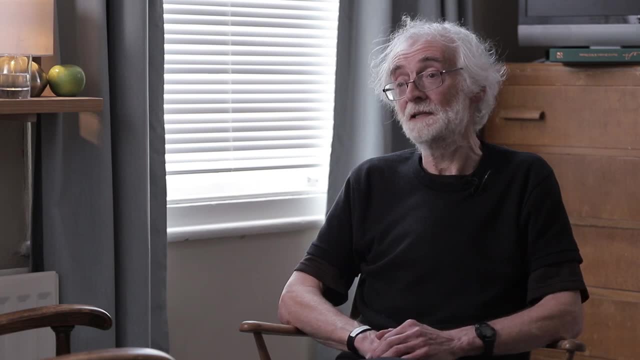 I can go zero, one minus one, Two minus two and so on, And all the integers appear sooner or later in that list. In the same way, you can do this with the rational numbers, But you cannot do it with the real. 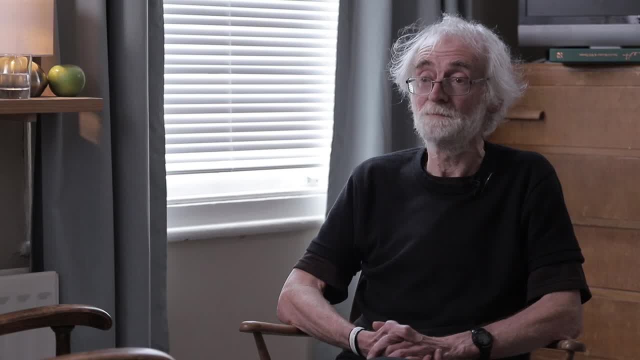 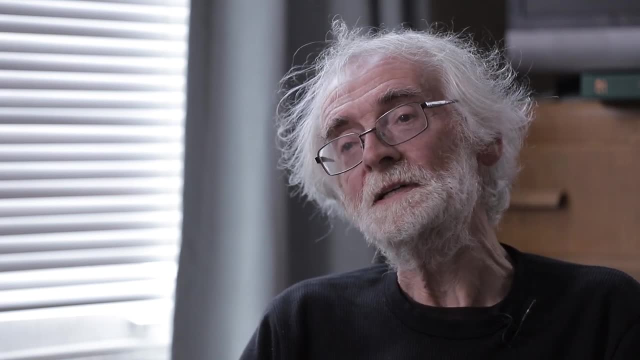 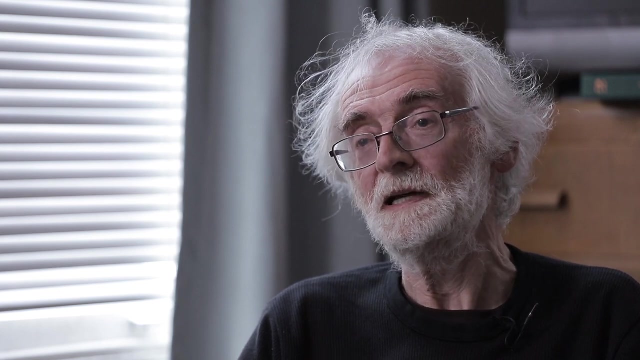 numbers. There are too many of them to form them into a list. In a similar way, there are too many subsets of the natural numbers to form them into a list. We say that they are two. They are uncountably infinite And I will try to prove this to you. It's a slightly 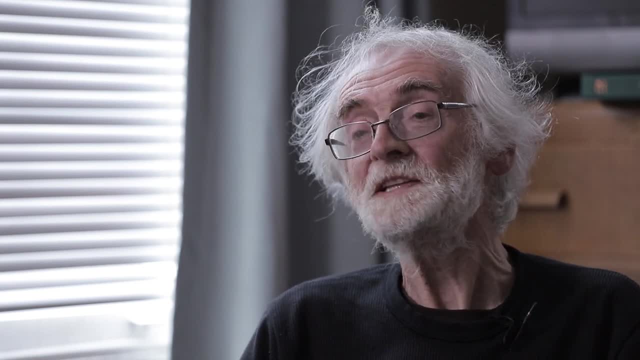 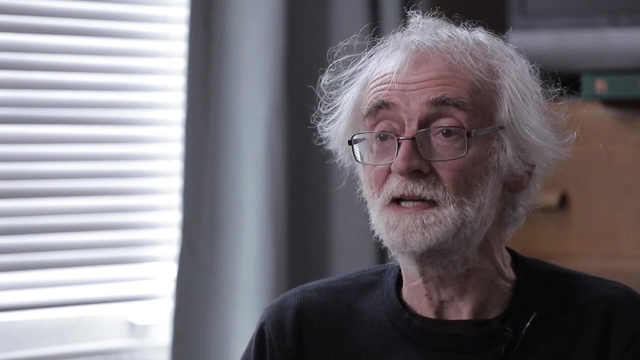 tricky argument, so please pay attention. Let's suppose that we could form all the sets of real numbers into a list, So there's a first set, a second set, a third set and so on. For instance, we could have the even. 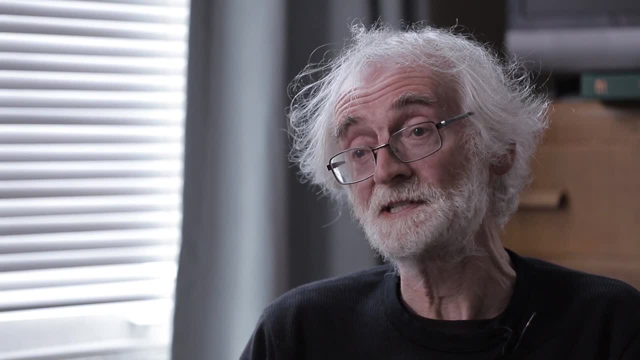 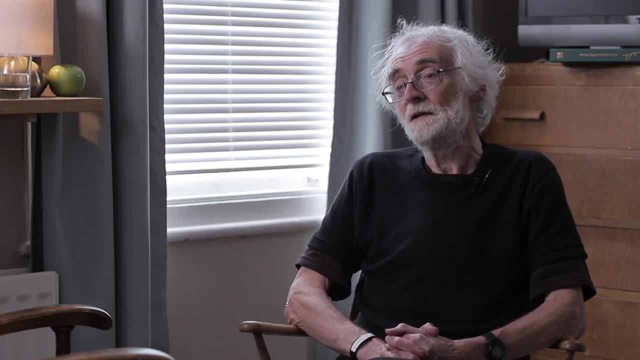 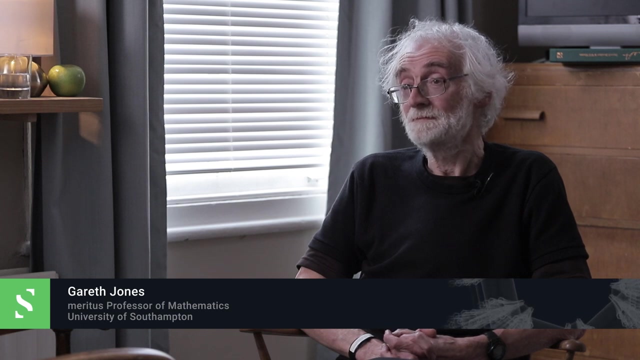 numbers as the first set, the odd numbers as the second set, the prime numbers as the third set, and so on. Now let me define another set of natural numbers. I'll call it S. It consists of all those numbers n which are not members of the nth set. I'll say that again: S is the set. 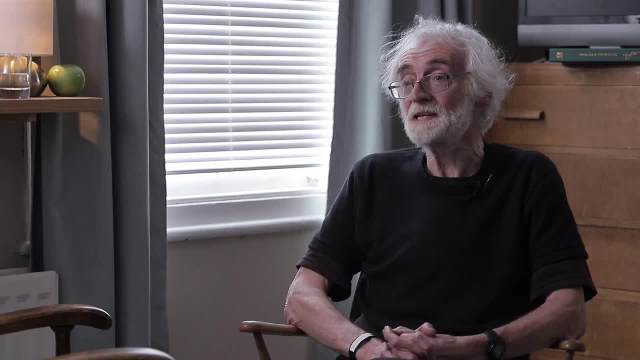 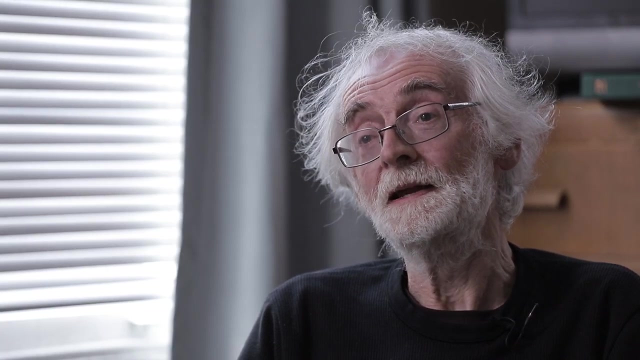 of all integers n which are not in the nth set S n. Now, if we have listed all of the subsets, then that set S that I have described must appear in the list. So it must be S n for some n. And now we ask ourselves: is n a member of this set S? If it is, then because? 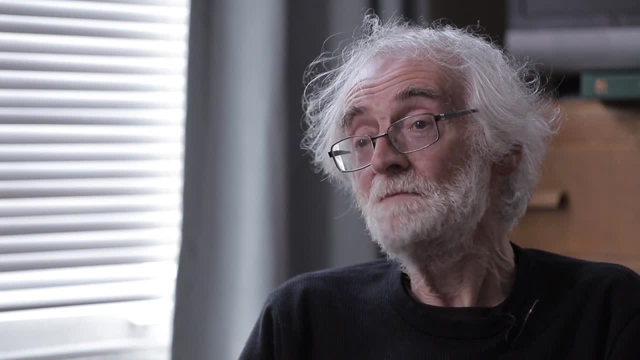 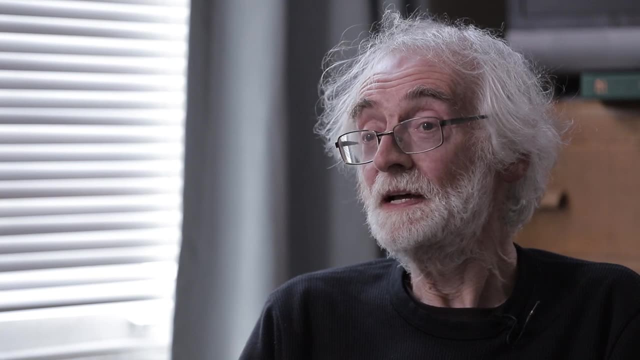 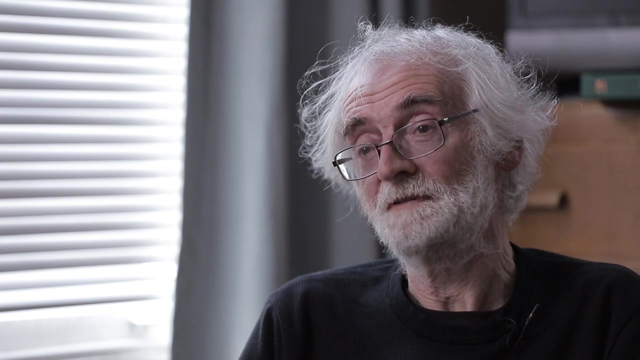 S equals S n. n is a member of S? n, But that means it's a member of S? n And therefore, by definition of S, it is not a member of S? n. And if S? n is not a member of S? n, then it's not a member of S And by definition of S, that means that n is not. 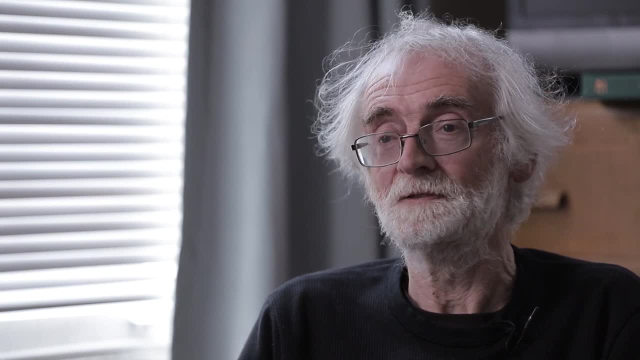 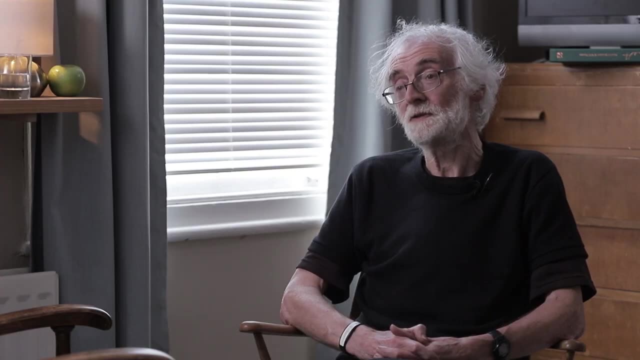 a member of S? n. So either way, we've got a contradiction. We've contradicted ourselves, And the contradiction must come from assuming that we could list all the subsets of the natural numbers. We cannot do this listing process. There are too many subsets of natural numbers to form. 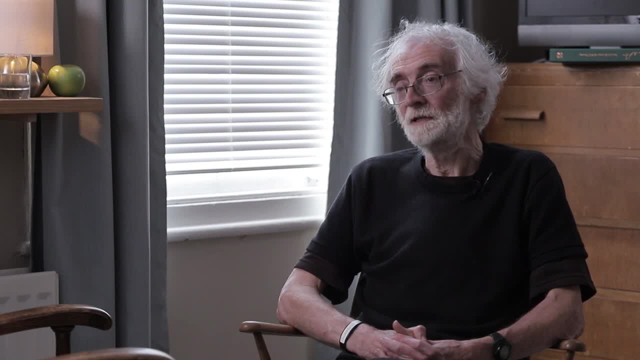 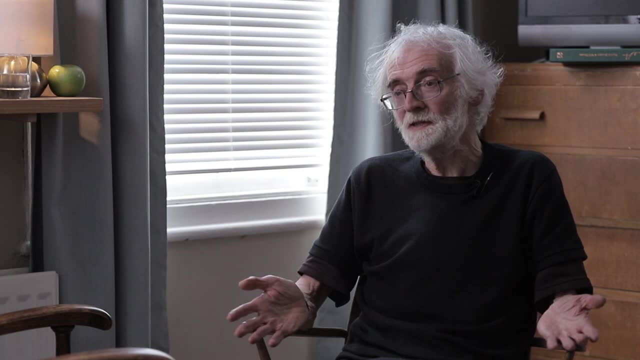 them into a list. They are uncountably infinite and that means that there are more of them than there are algorithms. We can write the algorithms in a list. We could just write them down in English and put them into dictionary order. just order them lexicographically. 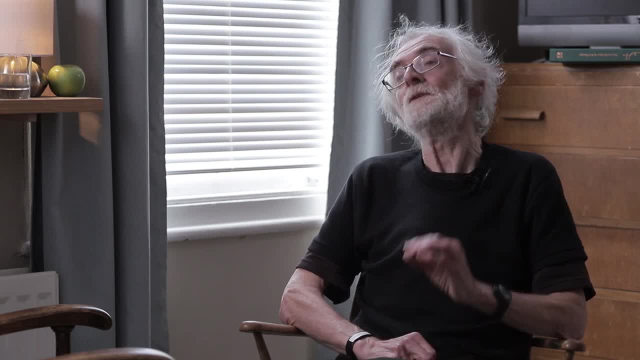 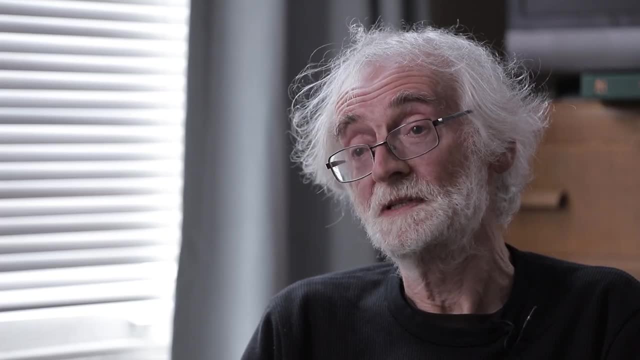 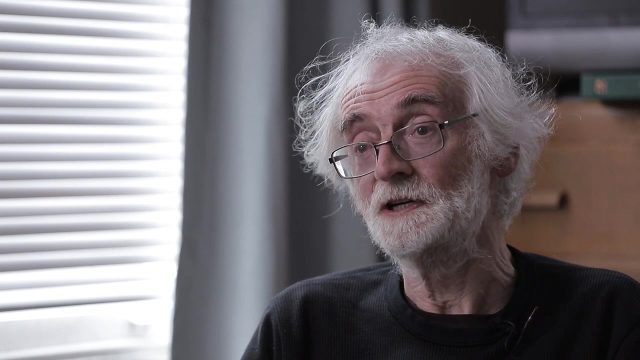 There's no problem about that. But we cannot list all the subsets of the natural numbers. We cannot do this listing process And therefore we cannot list all the decision problems, because for every subset of the natural numbers there is a decision problem: is this integer in that particular set? So 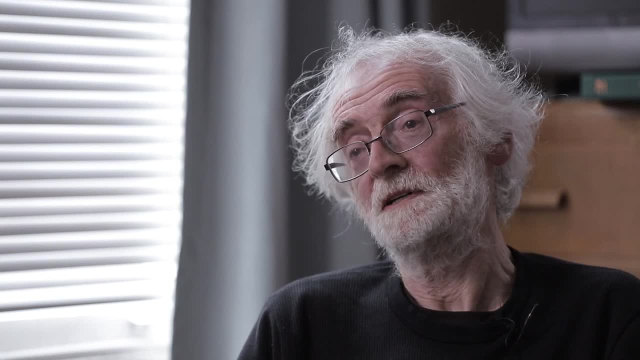 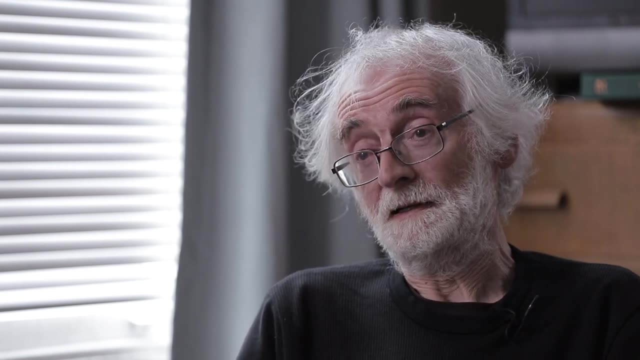 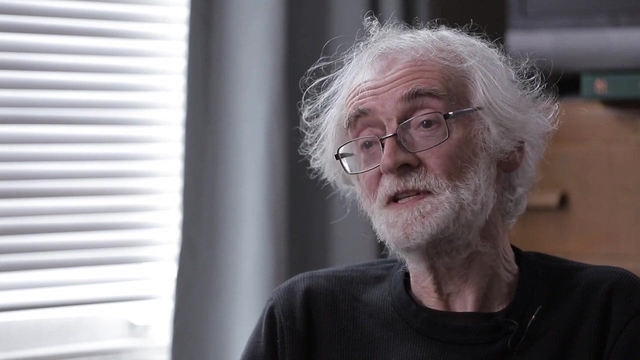 there are at least as many decision problems as there are subsets of the natural numbers. So I've tried to prove to you that there must be undecidable problems. But you'll be unhappy about that because I haven't given you an example. This does not produce. 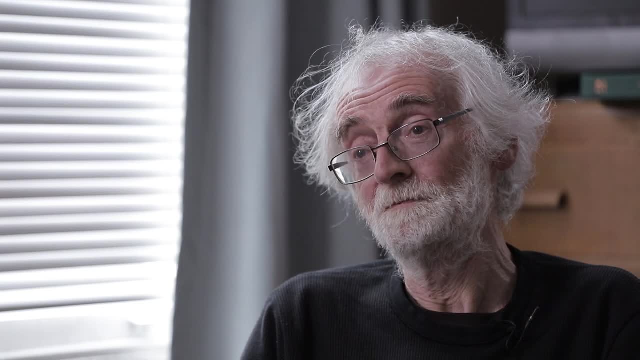 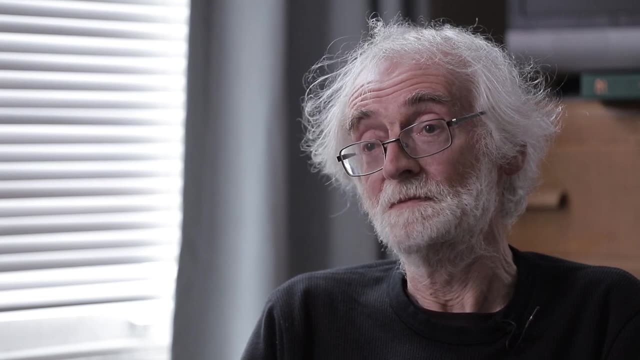 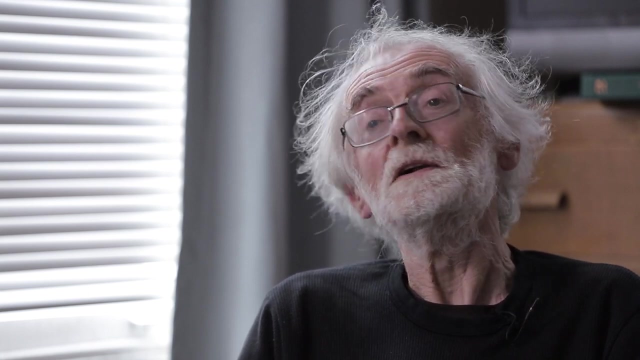 a specific example of an undecidable problem. What Turing and Church did was produce concrete examples of such problems, And I'll very briefly describe Turing's problem. He considered the halting problem. An instance of the halting problem consists of a pair. 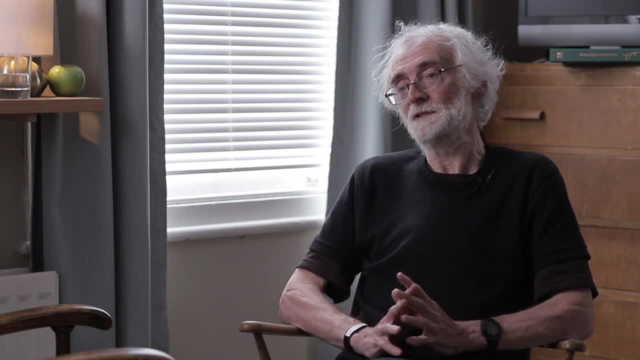 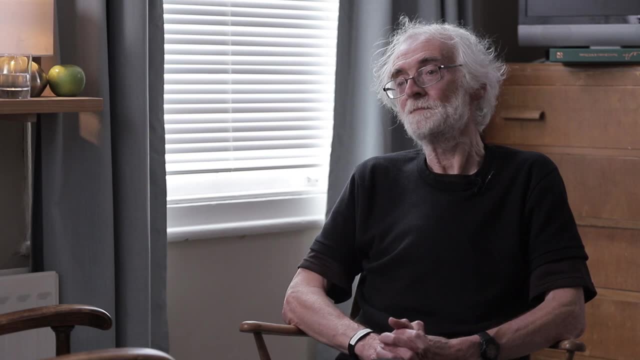 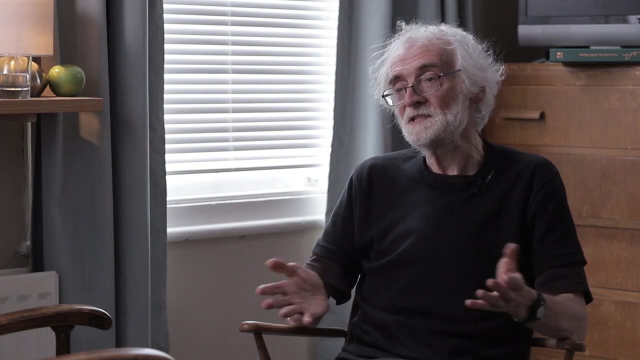 consisting of an algorithm and an input to that algorithm. And the halting problem asks: if you run this algorithm with this input, will it eventually halt or will it run forever? Let me give an example. Suppose the algorithm starts with an integer and the algorithm 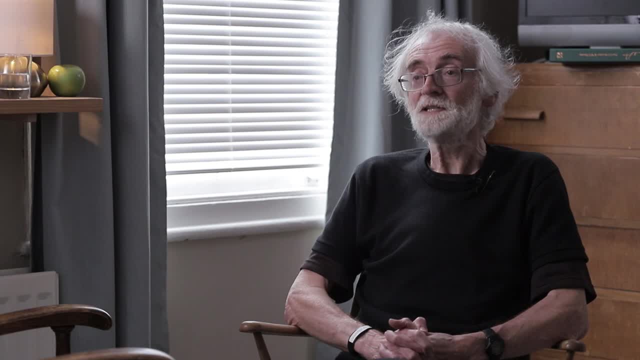 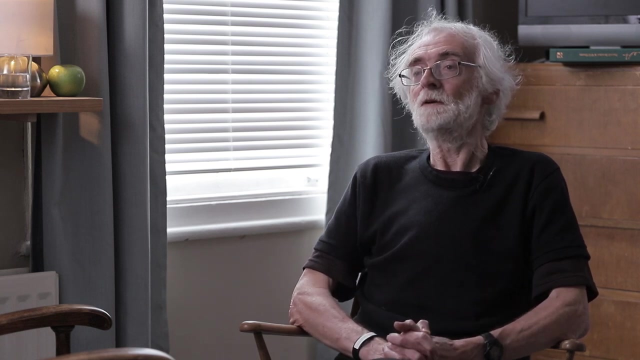 says: keep subtracting 1 until 0 appears and then halt. Now if I start that with an integer, say 3,, and run the algorithm, we'll get 3, and 2, and 1, and 0, and we'll halt. 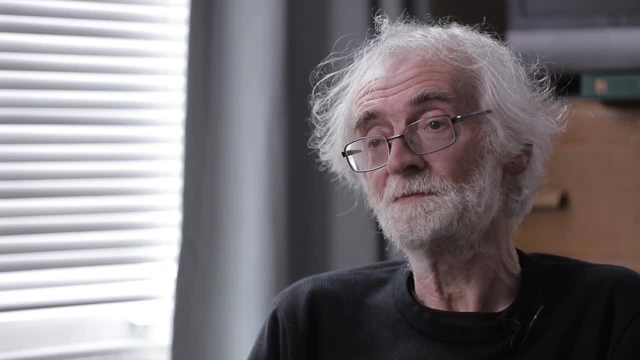 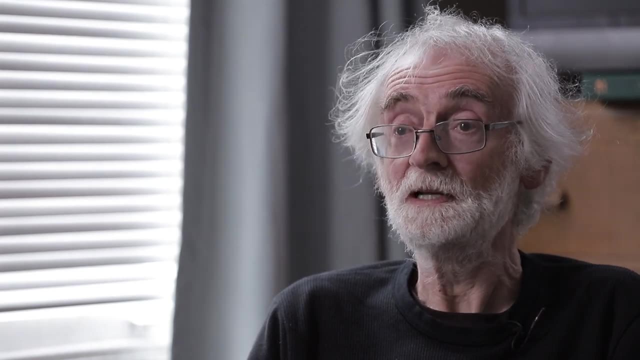 But if I start with a negative integer, say minus 1,, and run the algorithm, I keep subtracting 1, and I get minus 1,, minus 2,, minus 3, and it just goes on forever. We wait for 0 to. 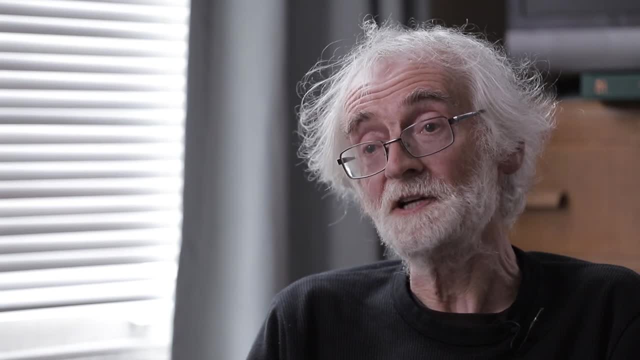 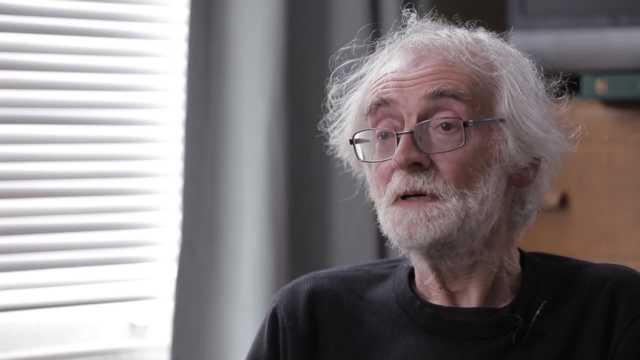 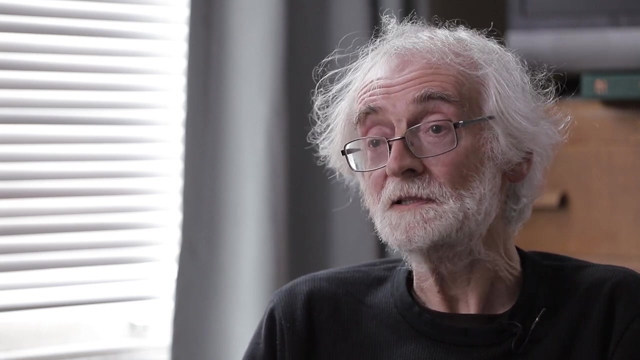 appear and it never appears. So the algorithm does not halt with that particular input. You could say we can solve this problem by just taking the algorithm and the input we are given and running the algorithm with that input and waiting to see what happens. Well, 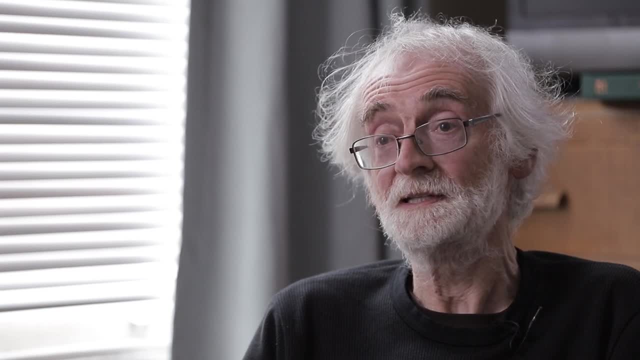 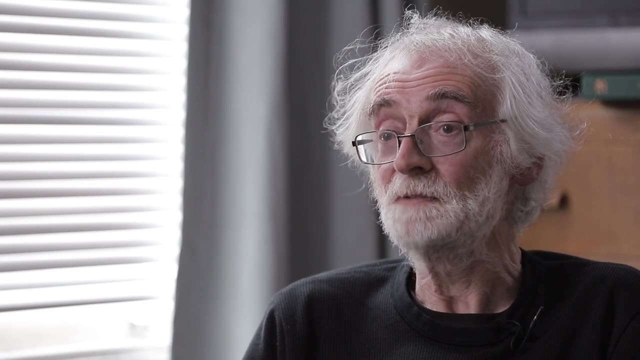 if the algorithm halts, we will see it halt and we will get yes as an answer. But if the algorithm does not halt, it will simply keep on running and we will be waiting for something to happen and we will never get a negative answer. 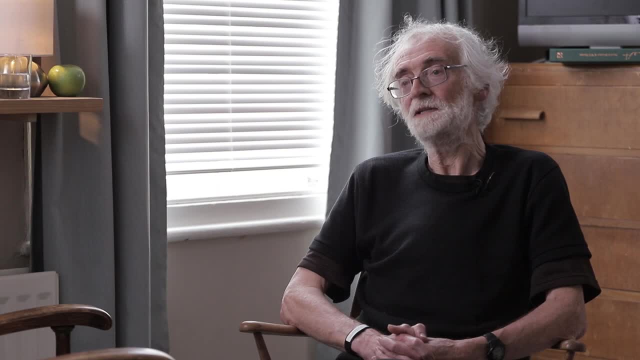 So simply running the algorithm is not adequate. It doesn't always give us an answer, And Turing was able to prove by a rather ingenious method of contradiction that there can be no algorithm which solves this halting problem. There is no uniform way of determining. 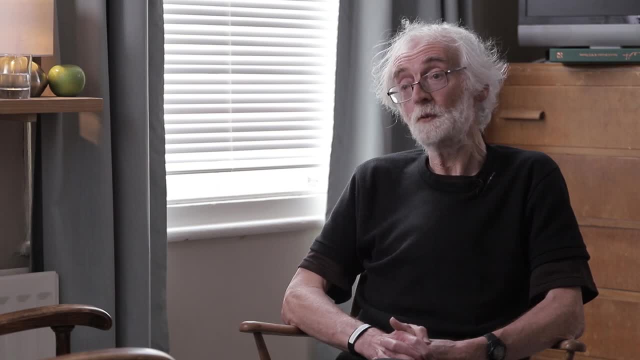 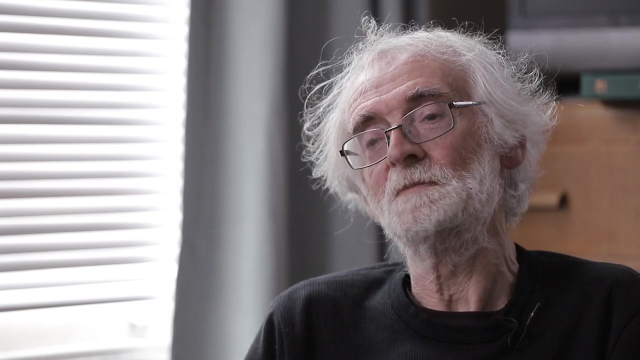 whether a given algorithm with a given input will halt. So the halting problem is unsolvable. I won't describe Chirch's undecidable problem. It's in algebra and it requires quite a lot of symbols to make it work. But what? these two examples of undecidable problems? 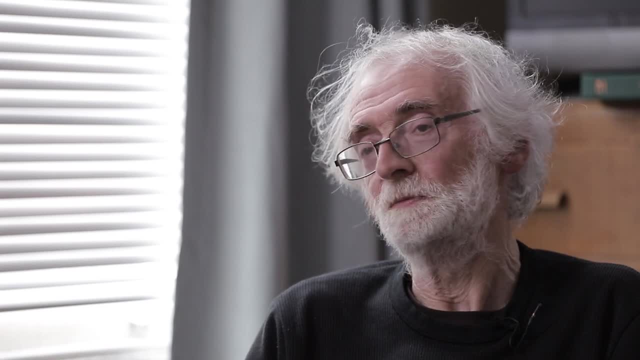 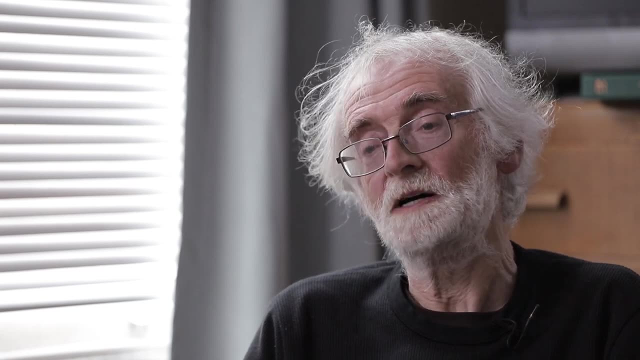 do is they give rise to other undecidable problems in other areas of mathematics, And since the 1930s mathematicians have found examples of important problems in algebra, in topology and in algebra, And therefore it is only to do so, particularly if you're. 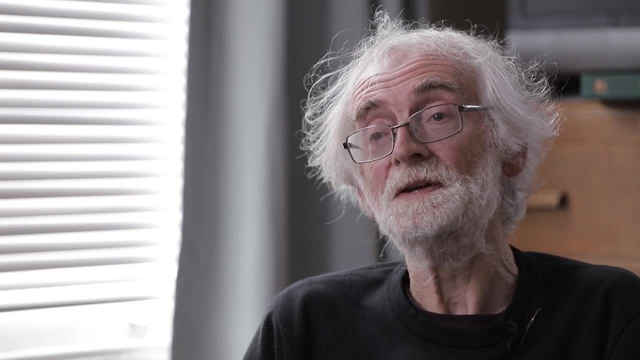 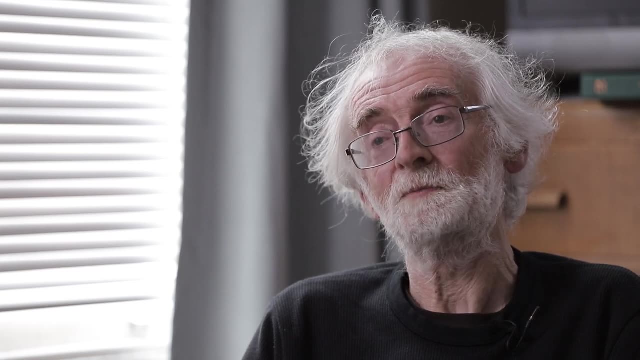 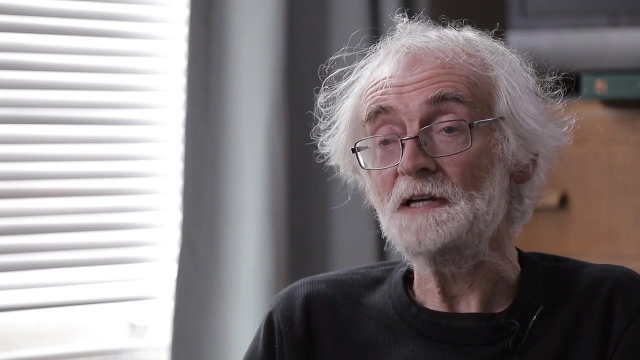 doing not-understanding problems in analysis and so on, which have proved to be undecidable. And I'll just finish with one specific example. This is Hilbert's tenth problem. In 1900, to celebrate the new century, Hilbert gave a talk in which he outlined a number of problems for 20th century mathematicians to 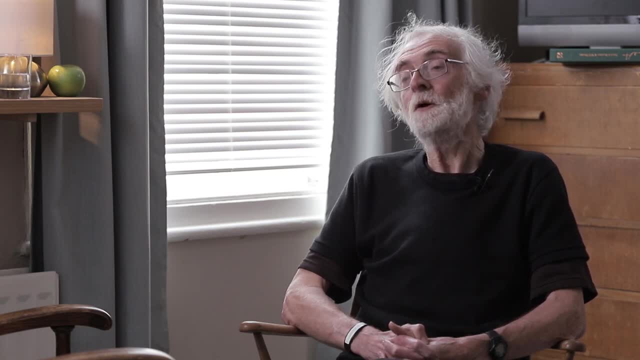 solve. Many of them have been solved, One of them, his tenth problem, was about Diophantine equations. These are polynomial equations with integer coefficients And he asked: if you're given a Diophantine equation, is there a solution in which the variables are all? 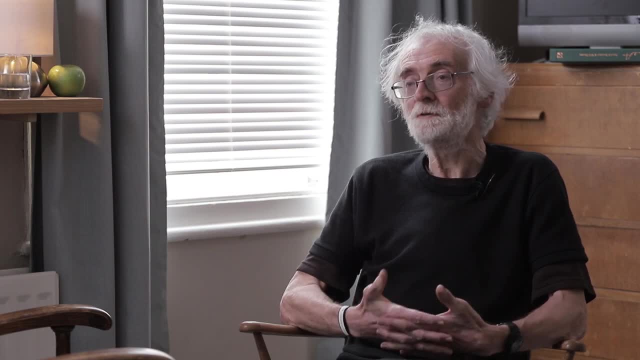 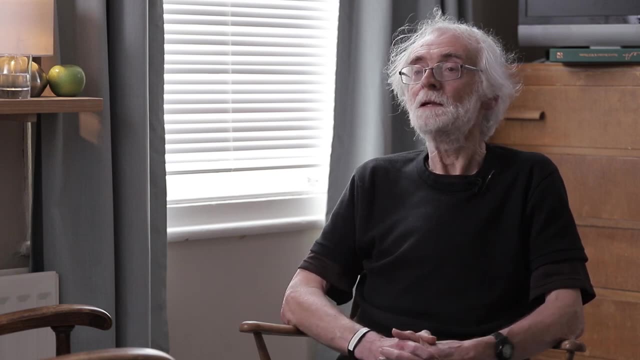 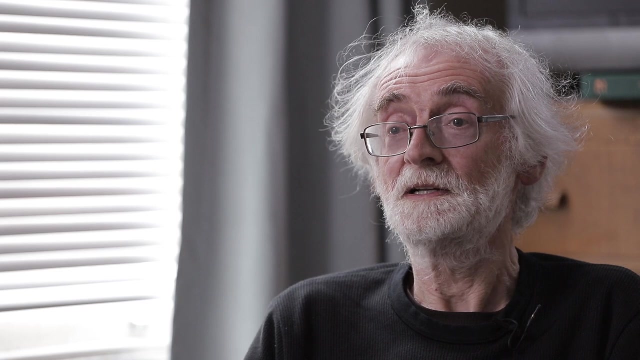 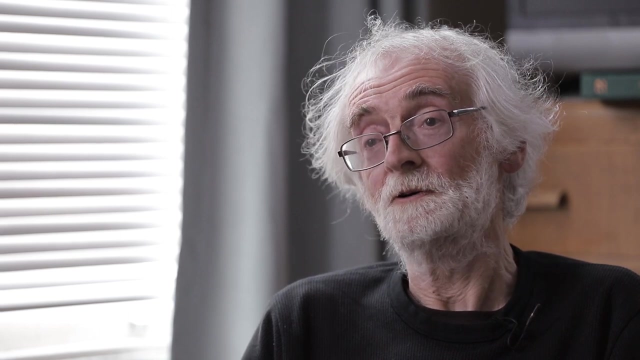 integers, And he wanted a uniform algorithm which would solve that problem. Here's an example. Let the equation be: X squared plus Y squared equal zero. It's easy to solve that. You can put: X equals Y equals zero. That gives you a solution in which the variables are all integers. 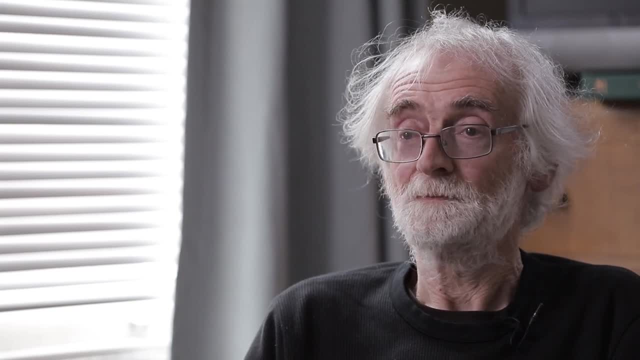 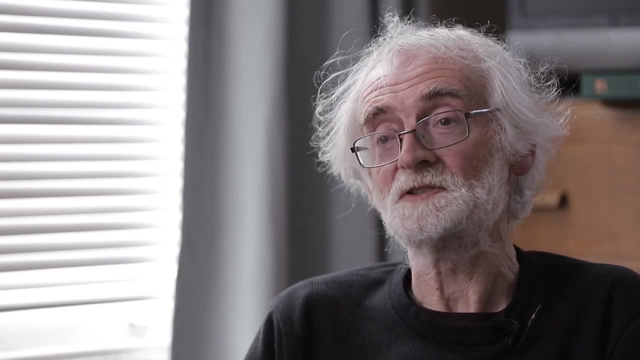 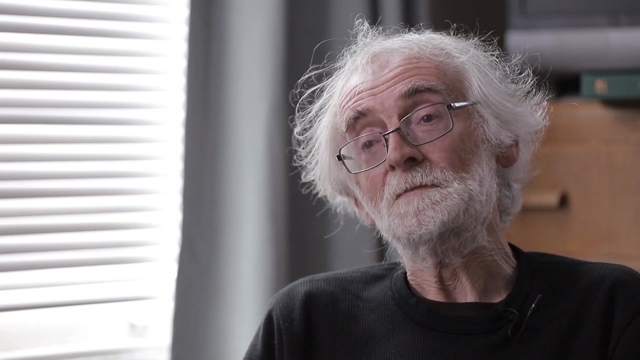 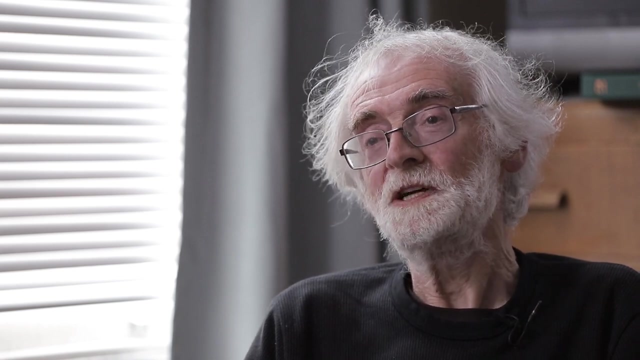 Now try: X squared plus Y squared equals three. You can solve it, but not with integers. There are no integers X and Y such as these at x squared plus y squared equals three. Just try it. That particular polynomial is easy to deal with, but in 1971 a Russian mathematician, Yuri Matyasevich, proved that there can be. 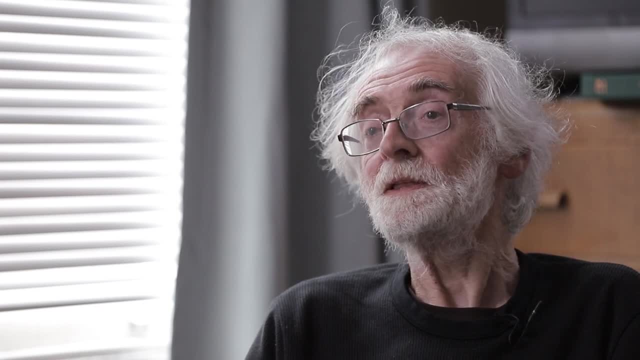 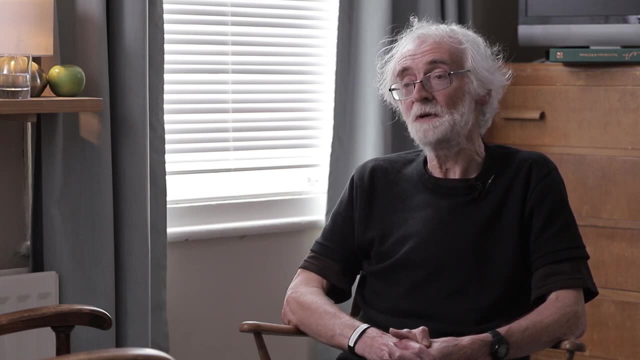 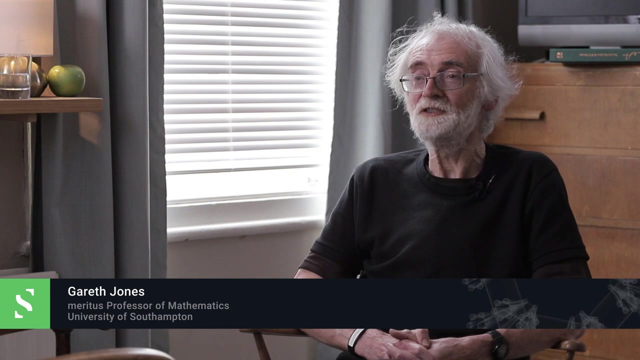 no algorithm which decides this question for all Diophantine equations. He did it building on earlier work by Davis, Putnam and Robinson. in the United States It was a time when cooperation between Russia and the West was not very good, but nevertheless, in subjects like mathematics, 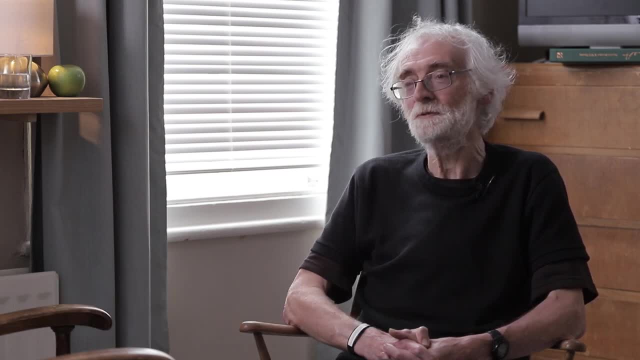 it's occasionally possible for people in different nations to talk to each other. What Yuri Matyasevich did? he used properties of the Fibonacci numbers to prove that there could be no algorithm to solve this problem. This is a very interesting problem. This is a very interesting problem. This is a very